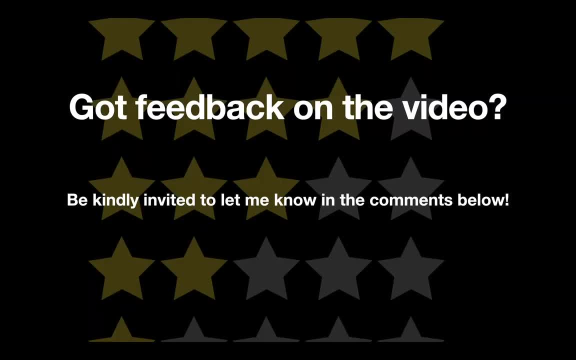 But very important, don't forget to come back If you have feedback. I am really looking forward to it, So let me know in the comments below. That being said, let's get started. We are starting with an orientation in RStudio. 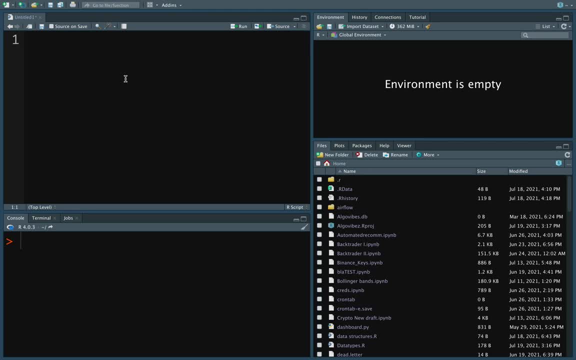 So I assume you installed both R and RStudio. I will link a resource how to install both in the video description. It is very easy to set up. So in the left upper corner you have the script part where you are writing R code in. 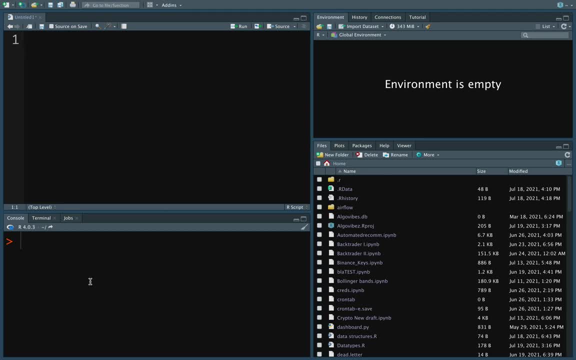 This code is executed in the console down below here. So let's take an example. If I just want to print out hello, I am writing that here and click on this run symbol. With that, this line, so line 1 is being executed and you will get the result of this line down below here. 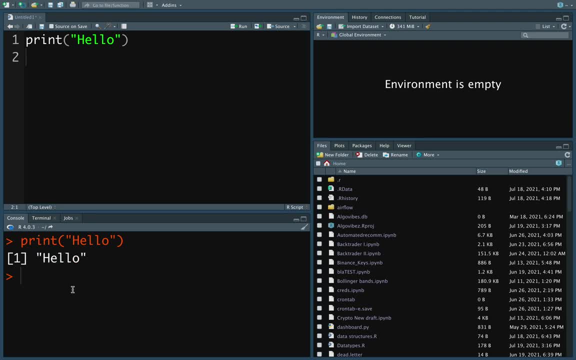 So just hello as an output. You can also directly type in the same printout statement here and you are getting the same result. Now let's move to assigning variables in R. First of all, let's get rid of that, And the first way to assign values to variables is to use the equal sign. 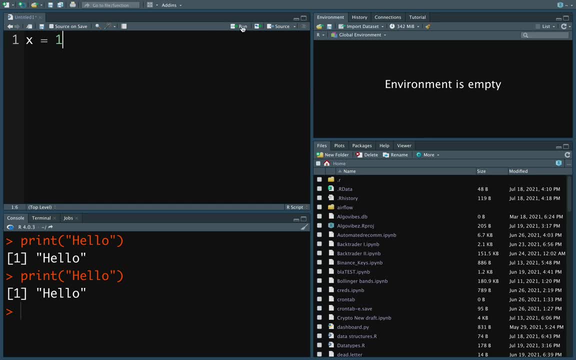 So if I want to assign 1 to x, I am just executing this cell, Or this line rather, And you are noticing that the x is appearing here and the value is stored to x also. So this is pretty handy here. Also, you can find out the value of x by just typing here: 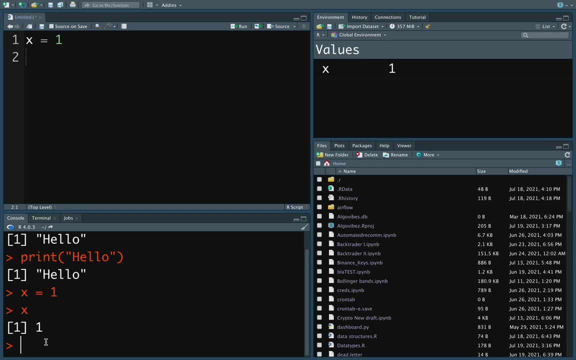 So now you see we are getting a 1 here, right. The second way to assign values to variables is using this one here. So let's assign 2 to y and execute this line. And now you see, 2 is assigned to y here. 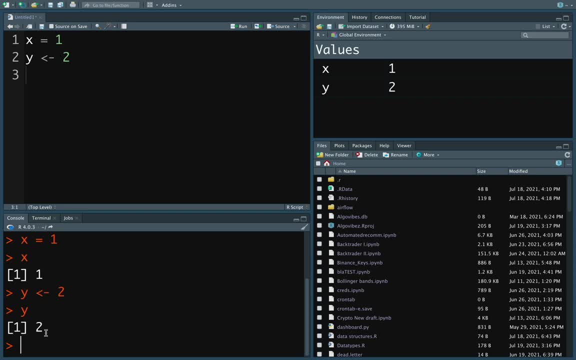 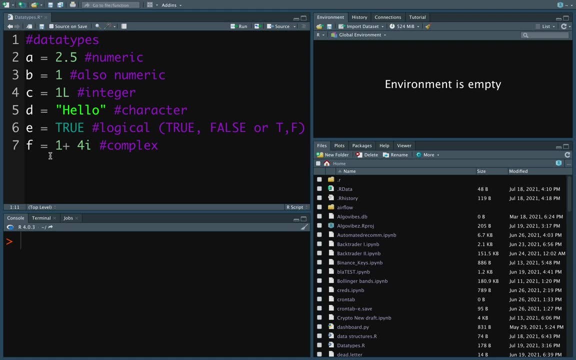 But you could also print out y here. Let's move on to data types. in R There are 5 data types which will be assigned to variables from A to F when executing this script. These purple values here are just comments which are not considered when executing this script. 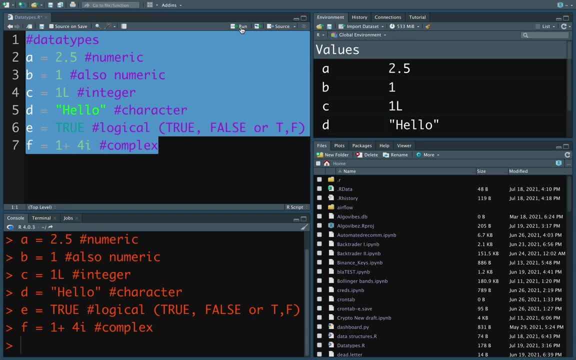 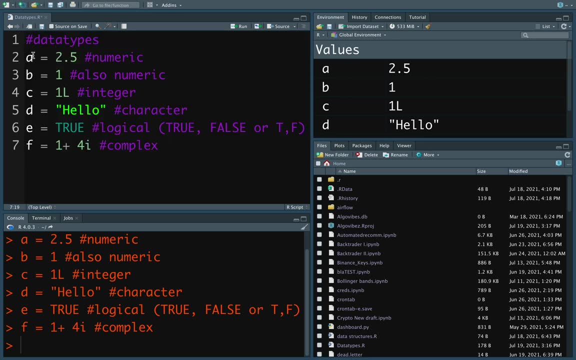 So let's mark that all and run this. And now we have assigned all variables and can take a look at them. So let's start with A, which is a numeric value. So let's print that out here And now. a very important function is the class function. 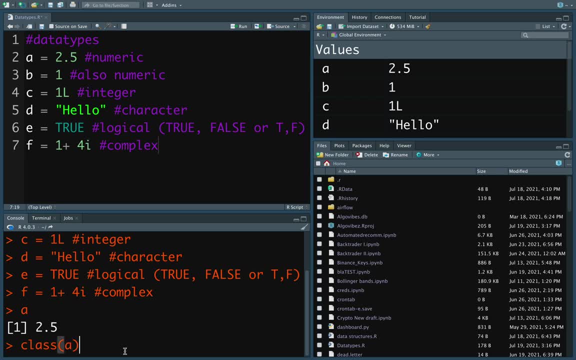 And if we are providing the A here, we are getting the data type of A. So we can just use class and then provide also a value of course. So you can also directly type in 2.5 and you are getting a numeric value. 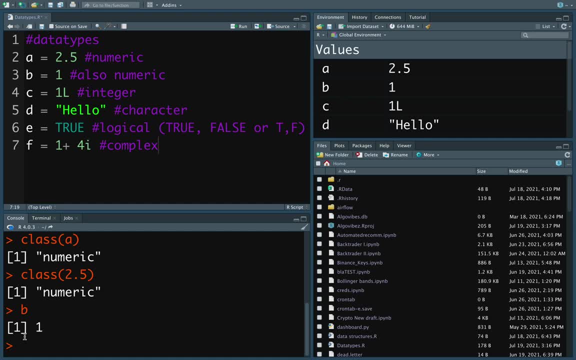 Second one, B, is a 1. And in mathematical terms it is an integer right, But in R it is also a numeric value. So you see that here, And this is kind of strange When you are coming from another program. 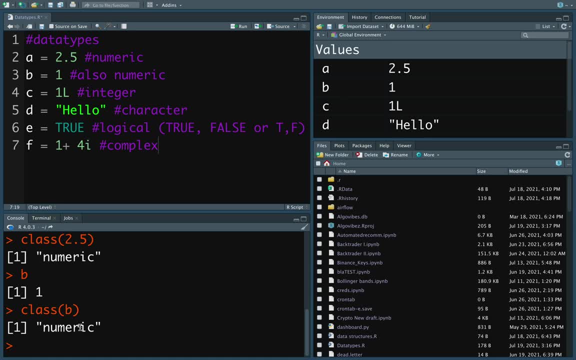 you are coming from a programming language, But it is how it is. So in R you are defining integers by using an L after the provided number. So C1L is an integer. So if we are printing out C here, we are getting a 1.. 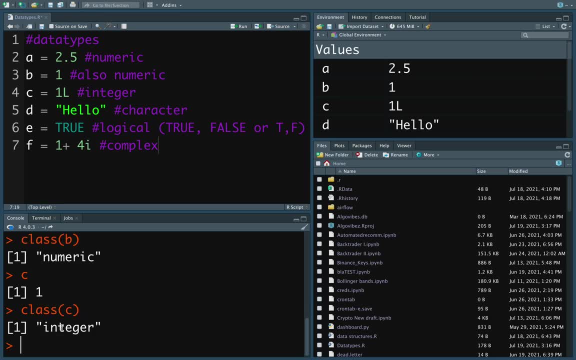 If we are taking the class function, we are getting the information that this is an integer, D is a character value, which are just text values. So if we are taking a look at the class function again, we are getting a character value here. 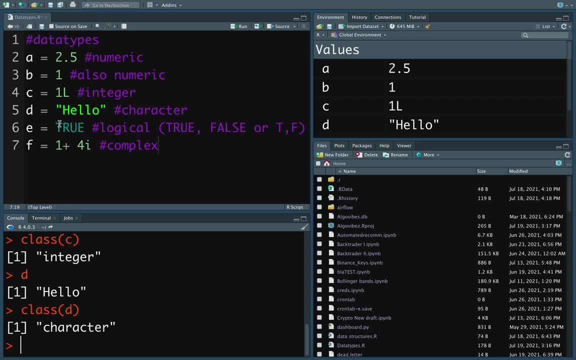 E is a logical value, or Boolean, which can take exactly two values: True or false. To save some time, you can also take T or F instead of true or false. So let's take a look at that. This is a logical value. 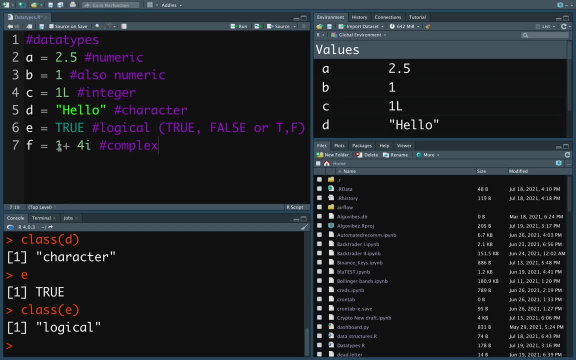 F is a complex value consisting of a real and an imaginary part, But I personally wouldn't see any use case where I would use that. but maybe you are. so here you are. Let's move on to operators. There are arithmetic and relational operators. 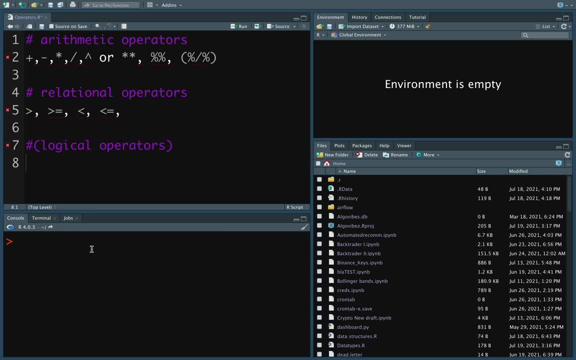 and also logical operators which I will use in the course of this video, but it doesn't make sense to cover them in this part. Explaining arithmetic operators is really straightforward. They are all usual math operations, such as addition 1 plus 1 is 2,. 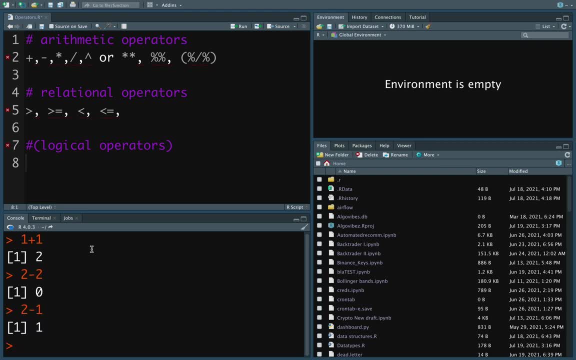 subtraction: 2 minus 2 is 0, or 2 minus 1 is 1, multiplication 2 times 2 is 4, division 6 divided by 3 is 2, exponent. we can take 2 to the power of 2, is 4.. 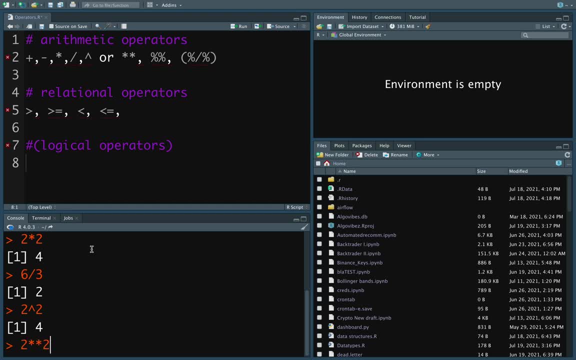 As an alternative, you can take 2,, 2 asterisks and 2,, and you are also getting 4.. So these are the two possibilities for the exponent And, last but not least, the modulus, which is calculating the remainder of the division. 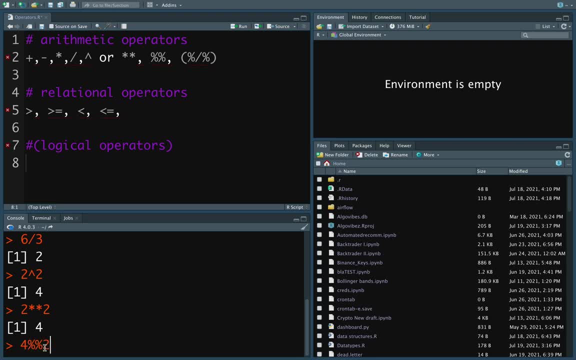 So let's take an example: if I'm taking 4, modulus 2, 4 is divisible by 2, then I'm getting 0 remainder here, right. But if I'm taking 5, modulus 2,, I'm getting 1 as the remainder of this division. 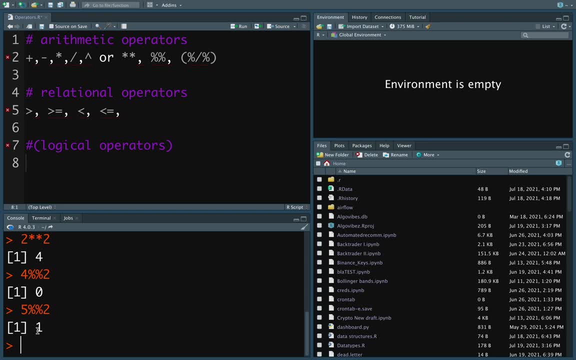 We will use that later to find out whether values are multiples of other values. So if I want to find out whether 15 is a multiple of 3, I can use 15, modulus 3, and I'm getting a 0. 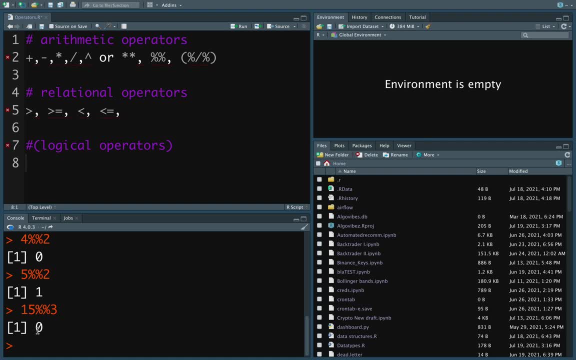 So 15 is a multiple of 3.. Last one would be an integer division, which I consider to be less important for beginners, so I'm skipping it. Now let's move to the relational operators, which are just telling you a certain relation between two values. 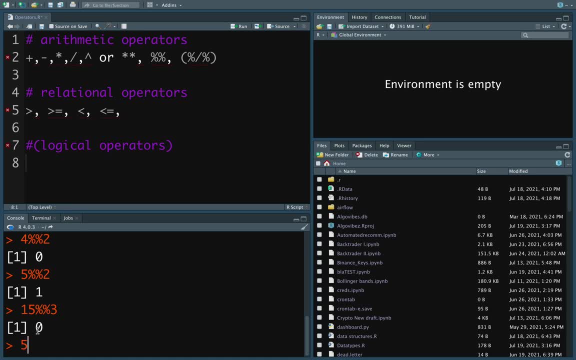 or even more than two values. But let's start easy. So let's take a look at 5, and then if it's larger than 3. And we are getting. we are getting an output here which is a logical or Boolean output, right? 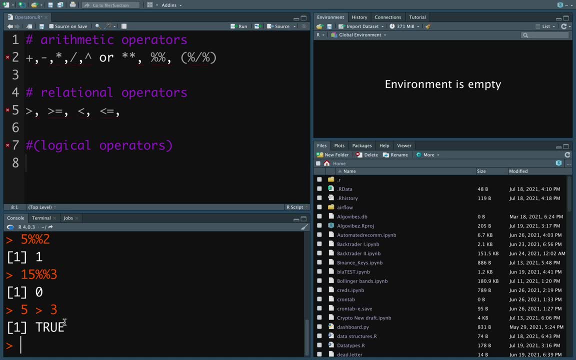 This is true because 5 is larger than 3, right. We can also take the larger than or equal to symbol. So we can take 5 is larger than or equal to 5.. And this is also true here, right? So, as an example, if we are taking 5 is larger than 5,. 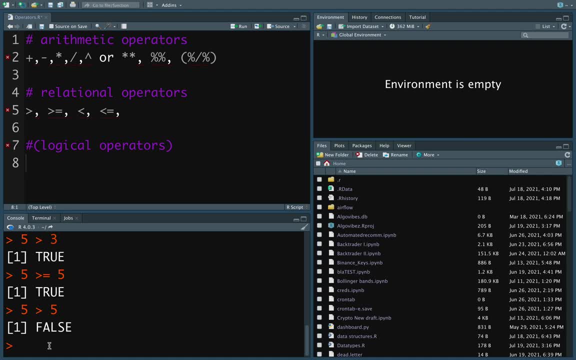 we are getting false here, right? This is the same for the other direction, so I'm not doing that here. But other important ones are equal to. So if I'm taking, let's say, 10 equals to 10, this is true. 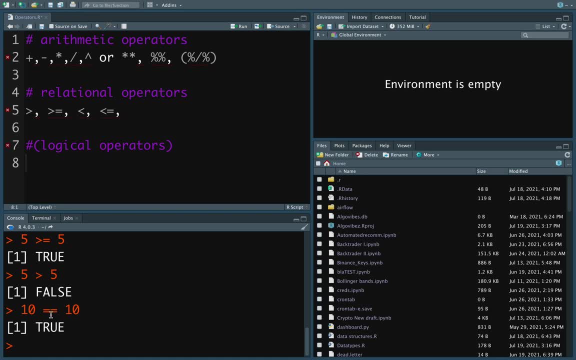 So this is just a double equal sign And finally we have the not equal to, which is, let's take: 10 is not equal to 5.. Then we are happy Having a true value here, because 10 is not equal to 5.. 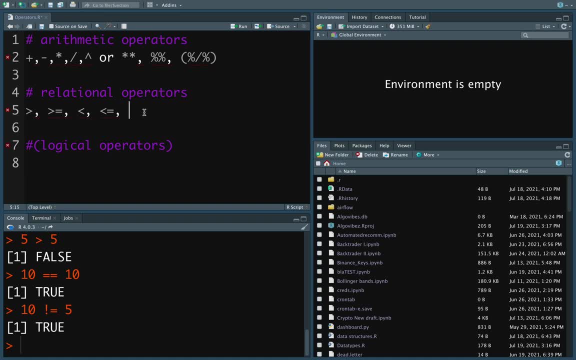 So I forgot to add them here. So let's add them equal to and not equal to, And that's it for operators. for now, Let's move on to create sequences. There are basically two possibilities to create a sequence. The first one, as you see here: 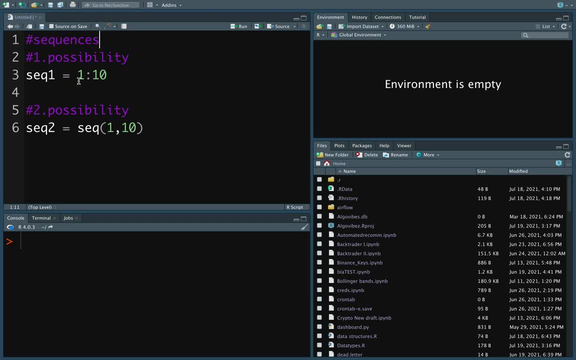 is using the colon operator and then specify the beginning of the sequence and the end of the sequence. So let's execute that and print out sequence 1 here And you see we are getting a sequence of values from 1 to 10 here. 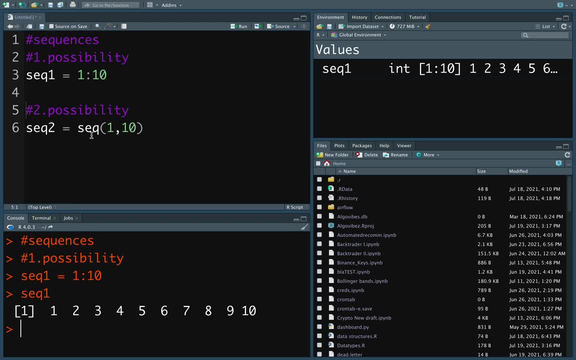 The second possibility is to use the sequence function from R, which is SEQ. So let's execute that and print out SEQ2.. And you see, we are also getting the sequence from 1 to 10.. This function is a bit more flexible than this one here. 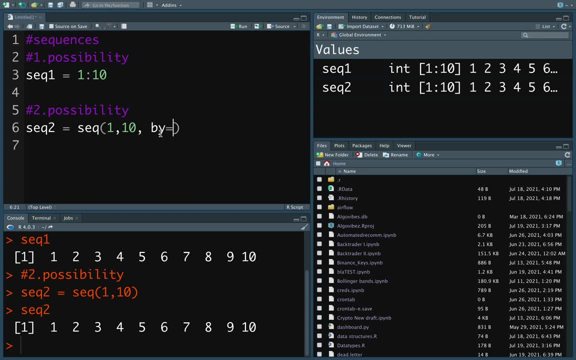 So you can, for example, define a step here using BY and then 2.. Let's execute that, And now you are only getting every second number printed out here, right? So 1,, 3,, 5,, 7,, 9.. 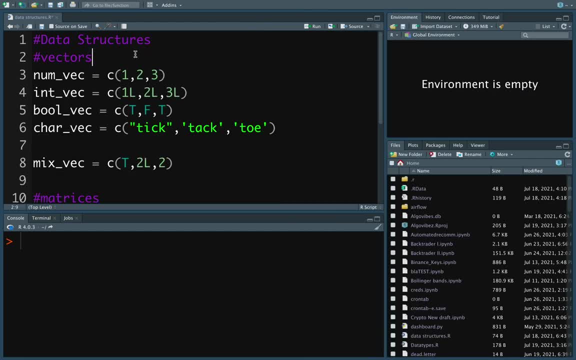 So let's move on to data structures and we are starting with vectors. So to create a vector, you are using C, open up parentheses and then comma separate the values you want to store inside this vector. So this is creating a numeric vector here. 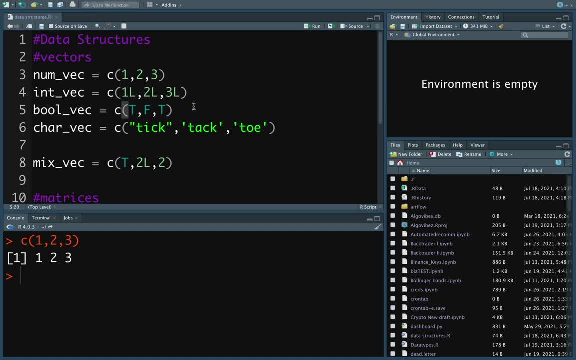 As you see here, I already created an integer vector, a logical or Boolean vector and a character vector. What's important, you can only store one data type inside a vector If you are trying to do the opposite thing. so you are storing different data types inside a vector. 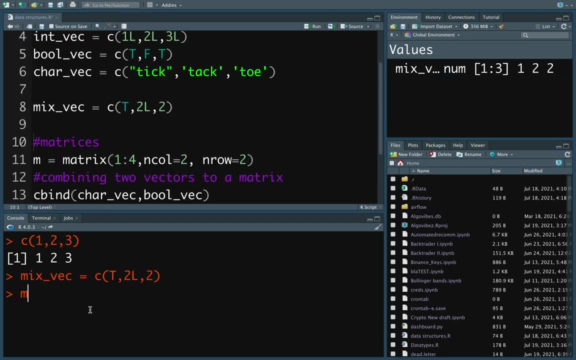 the following thing will happen. So let's execute this one here and print out mix vector. and take a look at the class function And you see we are getting a numeric vector here. So what is happening here? We have tried to create a vector. 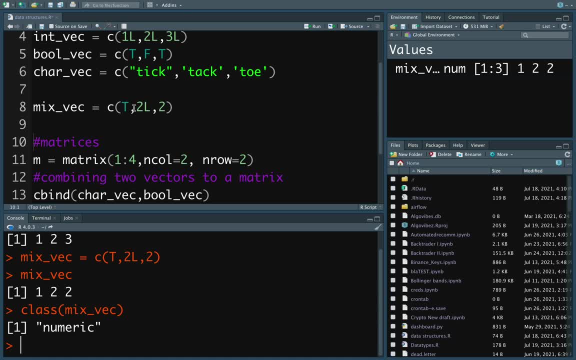 consisting of a Boolean value, an integer value and a numeric value, And R is transforming that vector into a numeric value. So the logic behind that is that R is taking the most flexible data type and is transforming this vector into this data type. 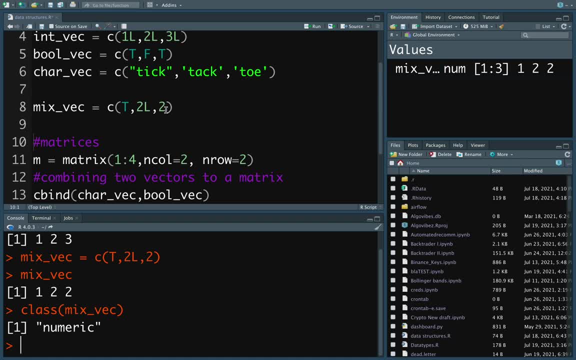 So the most flexible data type in R is the character, followed by the numeric value, followed by the integer value, followed by the Boolean value or the logical value. So if I would replace or add the character value here, so, for example, blah. 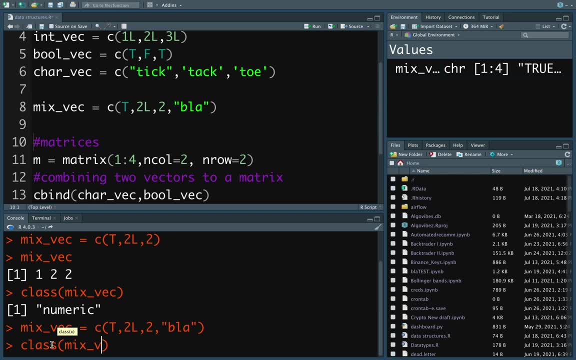 and execute that. take a look at the class now. I would get a character vector, because the character value here is the most flexible one, and the vector is transformed to a character vector. So, again, you can only store one single data type inside a vector. 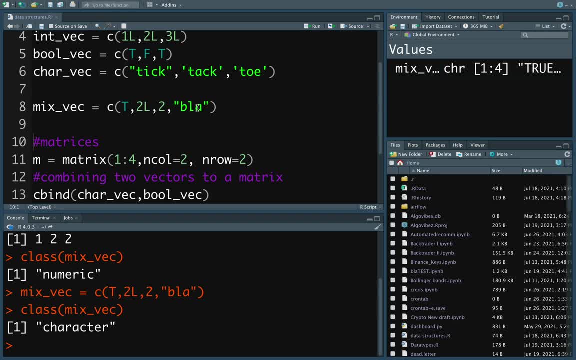 Now, to get more than one vector, more than one dimension, you can use matrices. So to create a matrix, you're just using the matrix keyword, then provide values you want to store in the matrix, and then the number of columns and the number of rows. 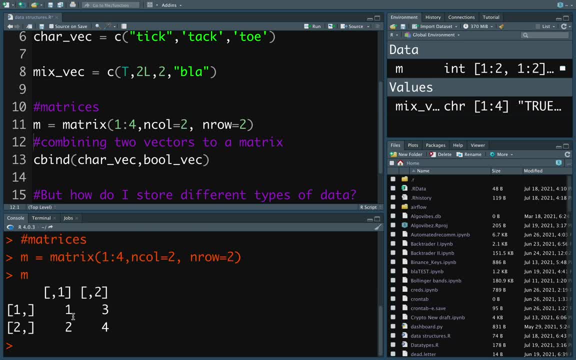 So let us execute that and print out this matrix. So I've created a matrix out of the sequence from one to four, with two columns and two rows, And the matrix is built like this. So one, two, three, four, right. 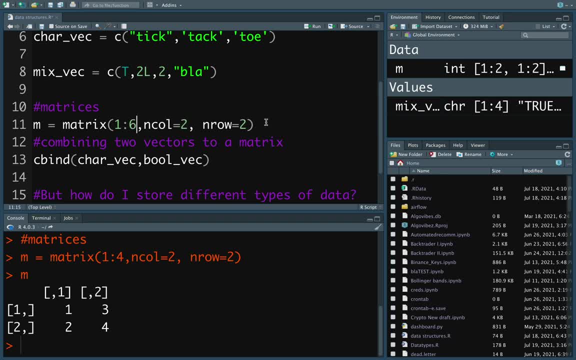 If I'm extending the sequence to six and print that out again, I would still get the sequence from one, two, three, four, as I don't have any more columns or rows where I can store the rest of the sequence. So five and six, right? 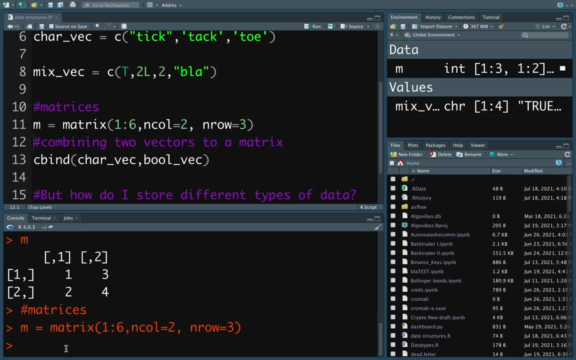 If I'm extending the matrix now by an additional row, you will notice that I got this: One, two, three, four, five, six, Okay, So how can I, let's say, create a column vector out of this? 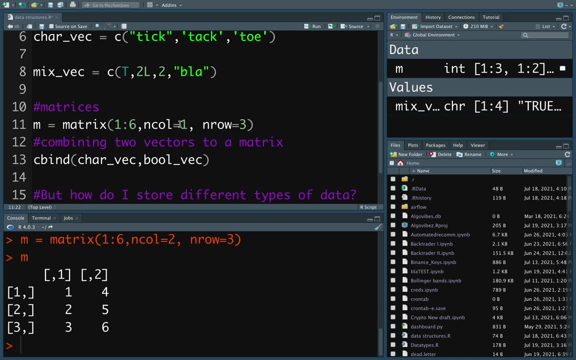 I can just use one column. Let's take a sequence of four here and take four rows, And with that I'm getting a column vector If I'm changing that. so if I'm taking four columns in one row, I'm getting a row vector, right. 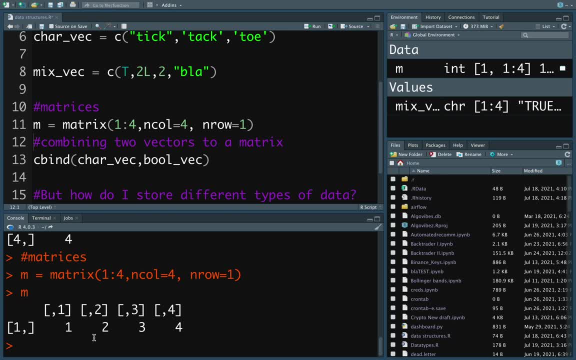 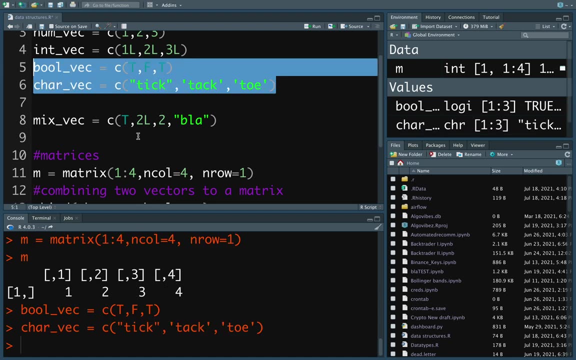 So I think you got the point right. I can combine two vectors to a matrix by using this C bind here. So first of all we have to quickly execute these, because they're not defined yet And if we are using C bind now, 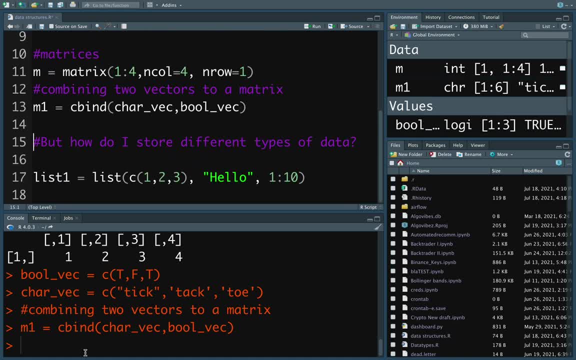 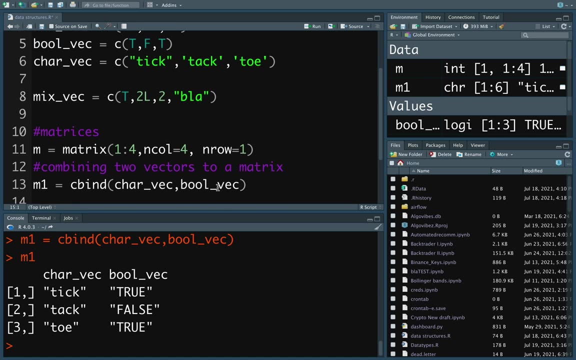 so let's just call that M1, execute that and print out M1,. we tried to combine the character vector- so this one here, tic-tac-toe- with a Boolean vector. this one here, tft. What is happening, as you see here. 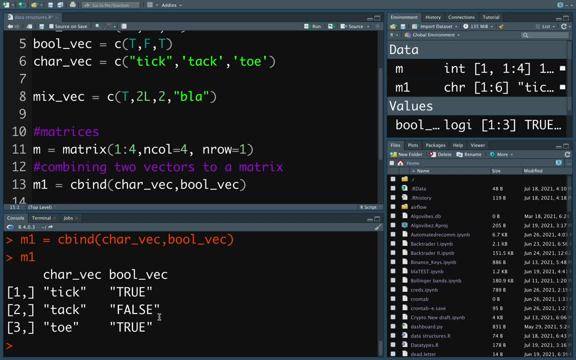 we are ending up with only character values, Also for the Boolean vector right Or the logical vector. So for matrices the same rule applies. You cannot store different data types inside a matrix right. What I also want to cover here at this point is indexing. 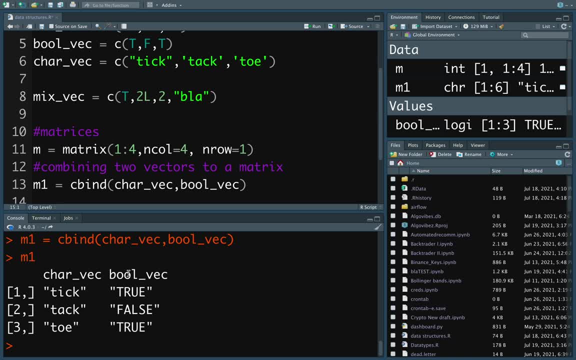 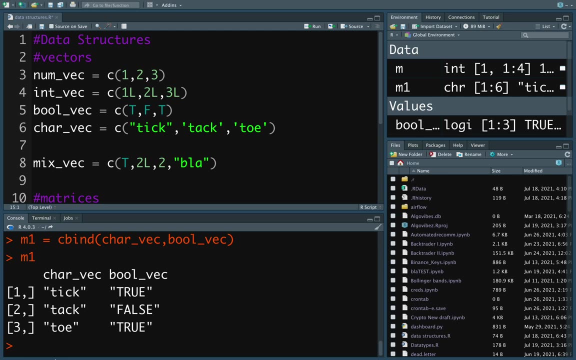 So what is indexing? I want to get a certain value out of a matrix or a vector And we are starting with vector indexing. So let's go a bit up and let's take a look at the character vector. So how can I get a certain element? 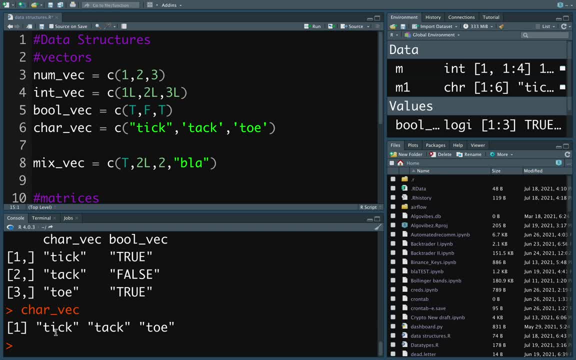 out of this character vector. So right now this might not make much sense to you to get a certain element, as you see all elements here, but you can imagine that there are vectors with millions of entries, right, And you want to know. 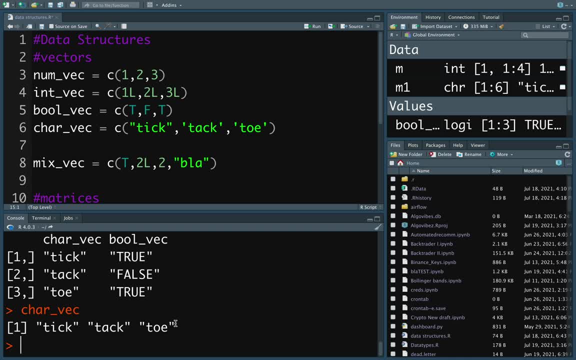 this value on an exact defined place. So to get the very first element from this vector. we are using squared brackets here, right, And different to Python. indexing in R starts at 1, right, So you might know that in Python. 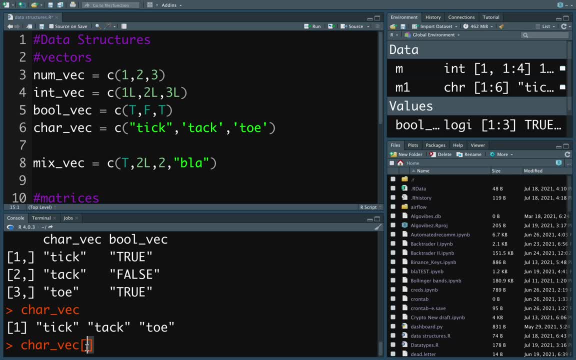 indexing starts at 0, but to get the very first element here out of this character vector, I'm just using 1.. And as you see, I'm getting tick here right. To get multiple elements, I can use 1 until 2.. 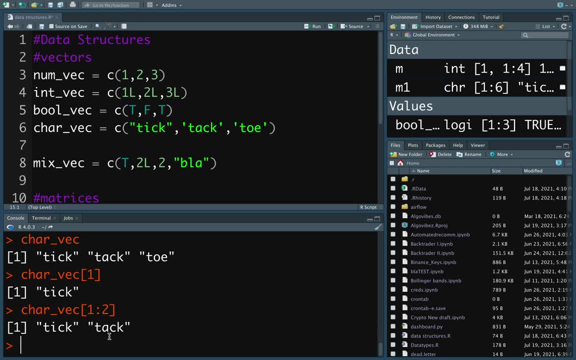 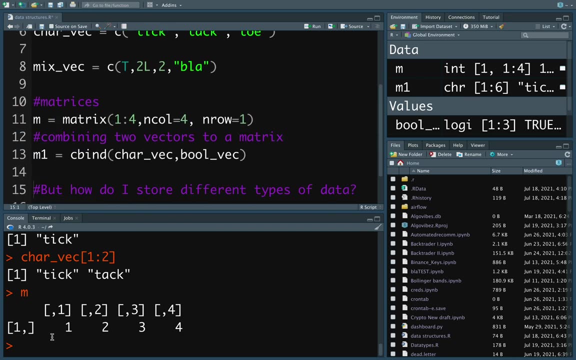 I'm getting tic-tac here right. So this is how indexing on a vector is working. Now let's take a look at our matrix again. Ah no, this is not good. I want to have a real matrix here. 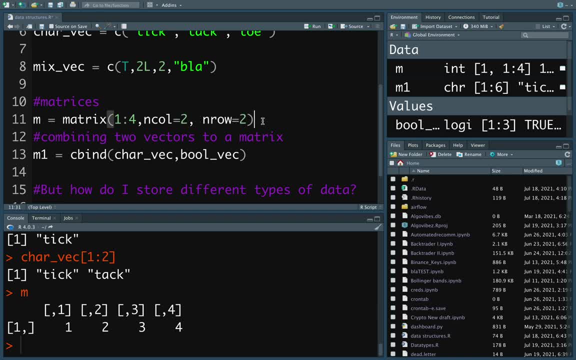 So let's just change that And let's keep this one. And indexing with matrices is pretty straightforward. So we are taking the matrix Again, open up squared brackets And if I want to have the first row of the matrix, I'm just using 1 comma. 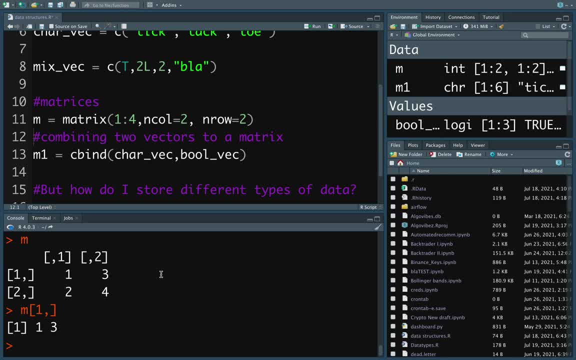 And you see I'm getting 1,, 3, right? If I want to have the first column of this matrix, I'm taking comma 1, and I'm getting 1, 2, as this is the first column of this matrix. 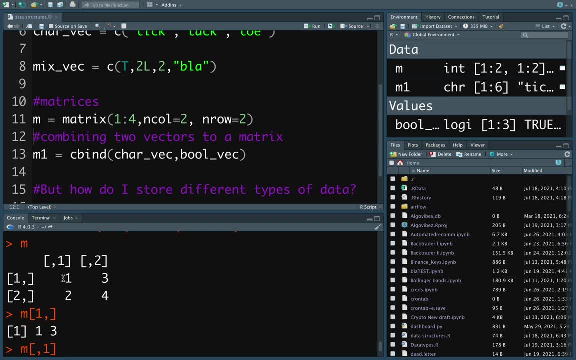 So if I want to have the first element, so the element in the first row, in the first column right, I'm just using m 1 comma 1, and I'm getting the very first element here, So the element in the first row. 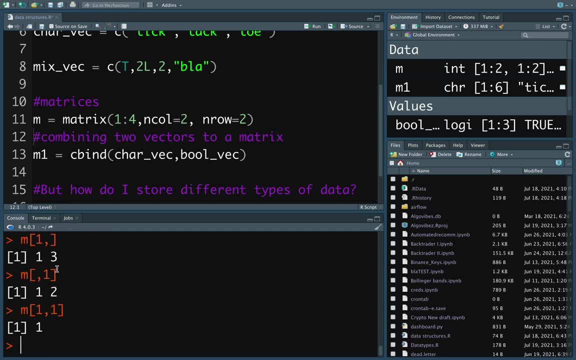 and first column right. So this is how indexing of vectors and matrices work. Okay, we got that, I think. But what if we want to store different types of data? We need something for that, right, And the solution for that. 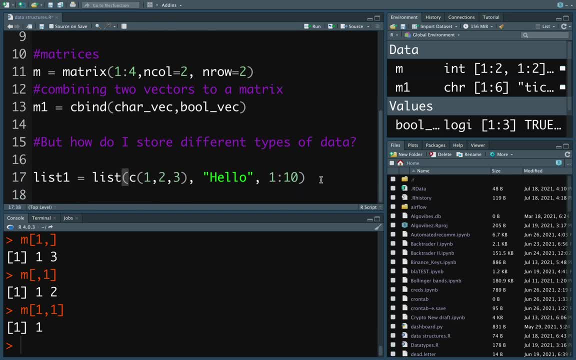 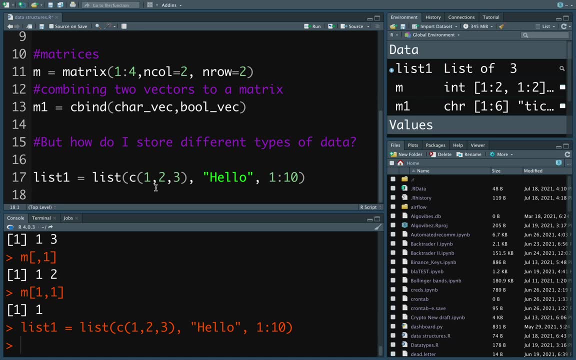 is using a list. I've done that here, so I'm executing that, And what I'm doing here is to use the list function of r. Then I'm providing a vector here, a numeric vector: 1,, 2,, 3,. 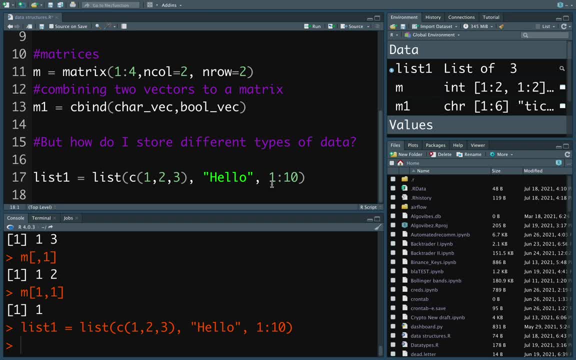 a character value and a sequence from 1 to 10, which is equivalent to an integer right. So let's print that out and take a look. And now you see, we're getting this list 1, with the first element as the numeric vector. 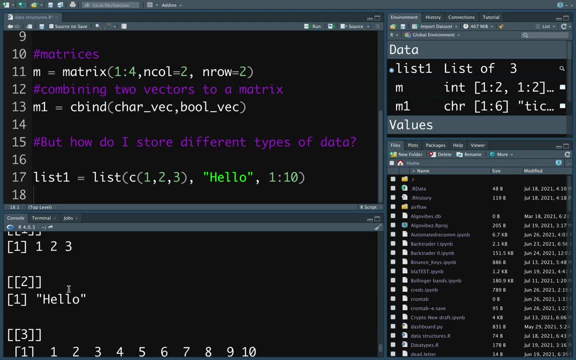 the second element as the character vector hello, and the third element as the integer sequence from 1 to 10.. So lists are enabling you to store different types of data. So how can I find out the types of data in a list? 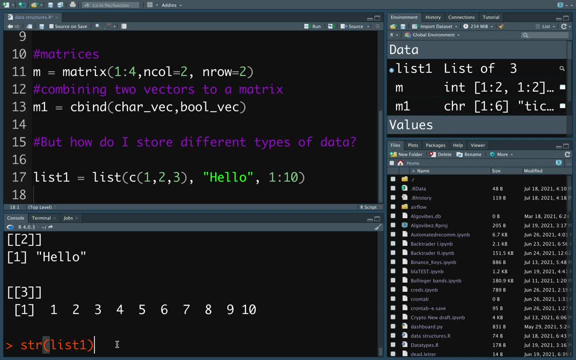 We can use the str function and provide list 1 here And you will see- and this is very handy. you will see, the first one is a numeric type, second one is a character and the third one- the sequence- is an integer. 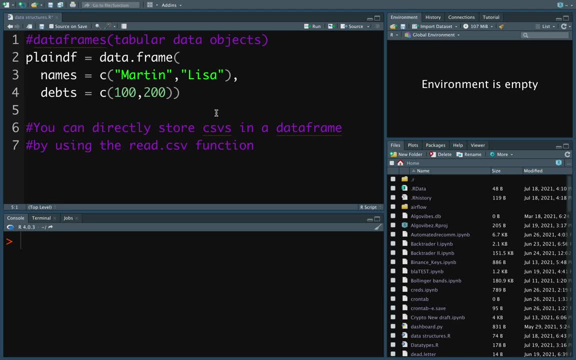 Okay, now let's get to probably the most important data structure, which are data frames. To create a data frame, you're using the dataframe function and provide the column name here and set that equal to the data you want to store inside this column, right? 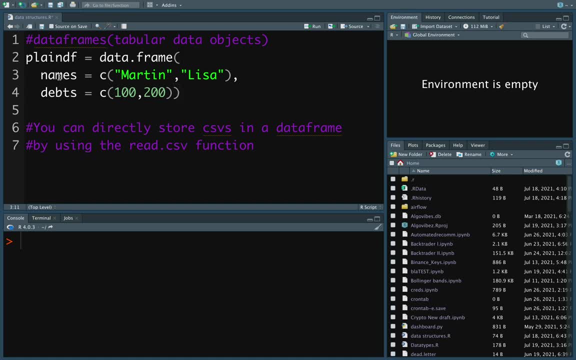 So in this case I'm just taking some names and I'm using a character vector here to store Martin and Lisa into the column names. Then I'm separating that with a comma and take the next column, which is that, and this is just the amount of money. 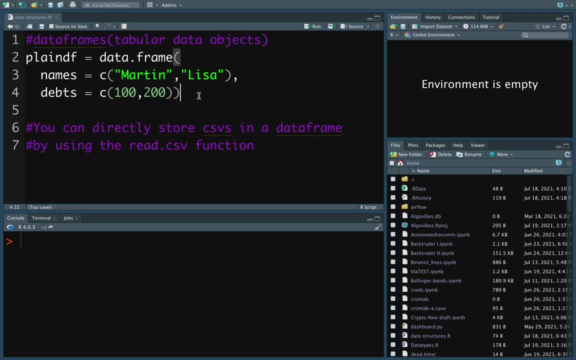 they are owing me right. So these are numerical values. So let's execute that and take a look at that. And now we see we have this handy data frame containing names and the amount of money they are owing me. What's special about data frames? now? 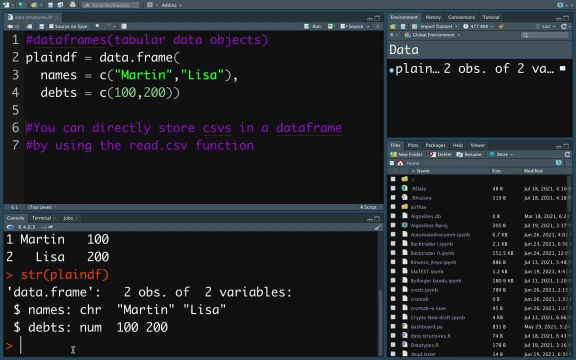 is. if we are taking a look at the types, we are noticing that the names are character values and the data are numerical values. So we can combine different data types. here Indexing with data frames is working exactly as it works with matrices. So if I want to get 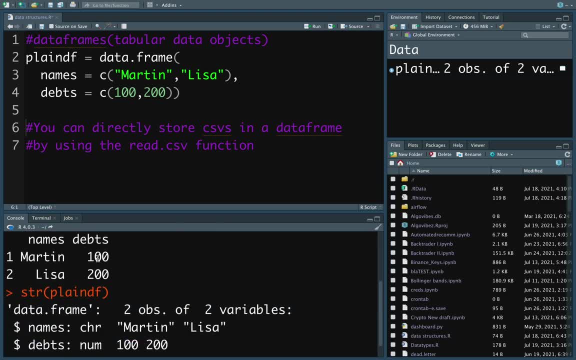 let's say only the depth. I'm just using plain df and use comma two for the second column and I'm getting the depth. And if I want to get the first value in the first row and column, I'm using one one and I'm getting Martin here. 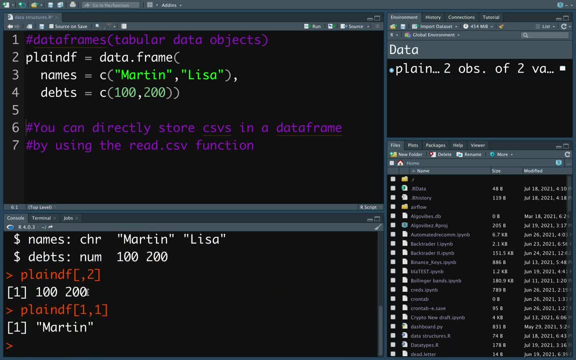 Right. So what is very, very important in R is the read CSV function. So if you're using the read CSV function and reading in a CSV file, then you are storing it directly in the data frame. So let's take an example for that. 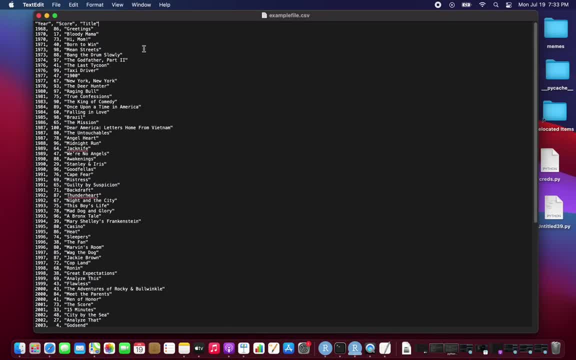 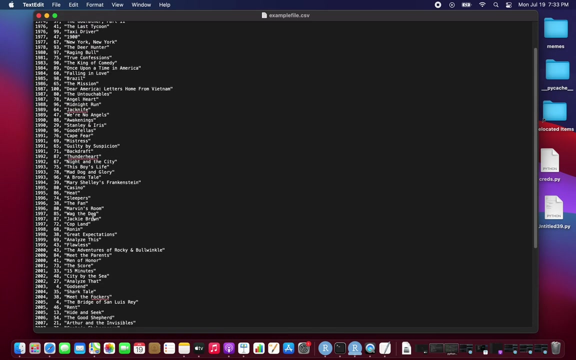 So I've just picked a random CSV file here. I think it's the Rotten Tomato numbers or, I don't know, the ratings for De Niro films, as far as I know Right. So these are the years, the score and the title of the film. 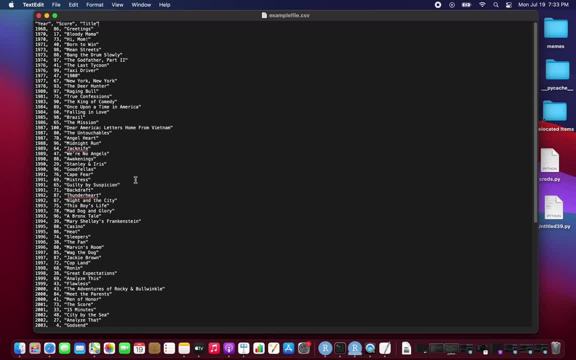 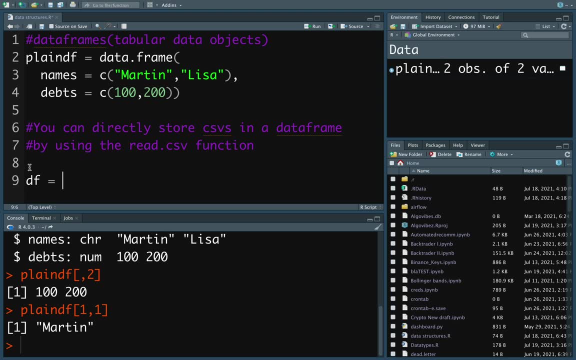 Right. So I want to read in this file, and that's actually pretty easy. So let's create a data frame. So this is just the variable where I'm storing it in And I'm using read CSV, And here I just have to provide. 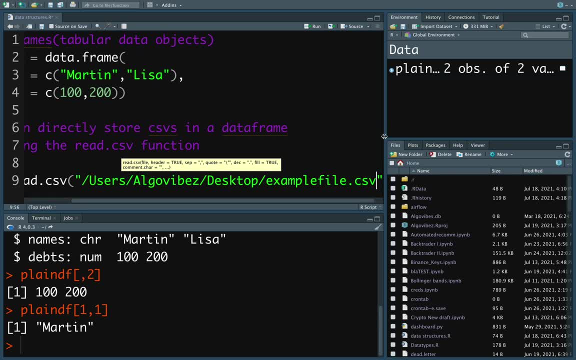 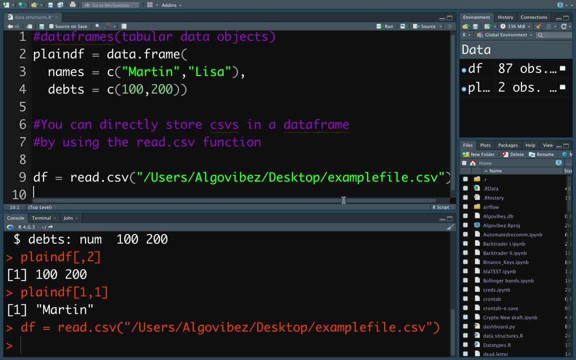 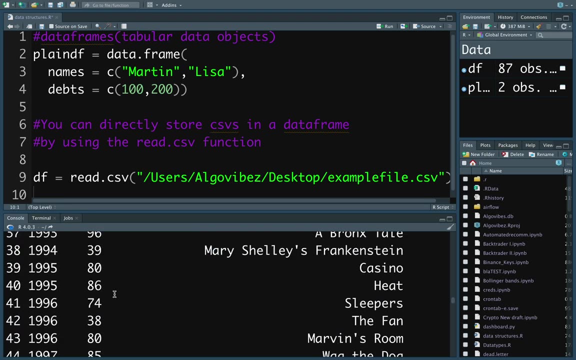 the path of the CSV file, Right? So in this case it's on my desktop, as you just saw, And we can execute that. And now take a look at the data frame. And now we see we are getting that, as you saw before. 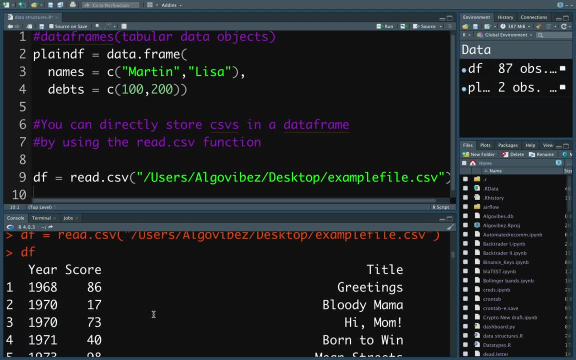 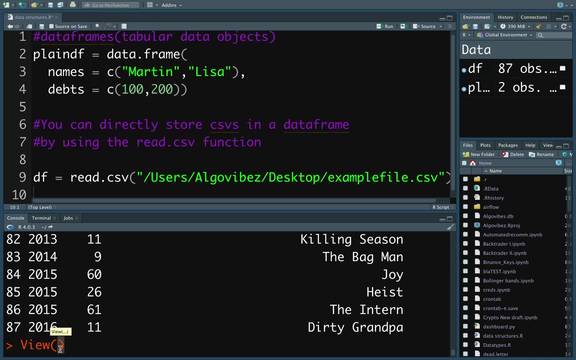 Right, And as this is not really lucid, I'm showing you a very, very useful function, which is the view function, And here you have to provide the data frame you want to view, And if we are doing that, we are getting. 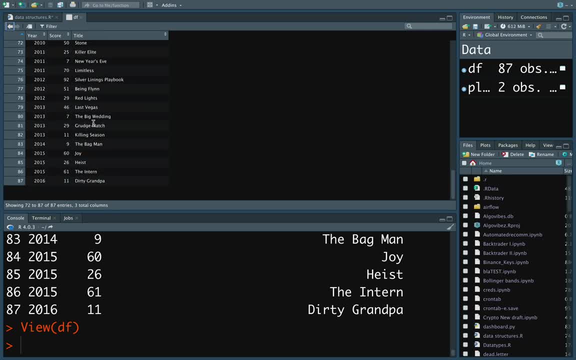 the whole data frame up here, Right- And this is totally awesome, Right- To just give you an idea of what you can do with data frames. So I'm not doing any data science stuff here, but just to give you an idea. if I wanted. 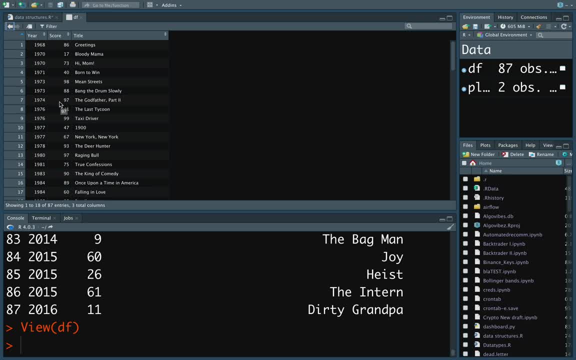 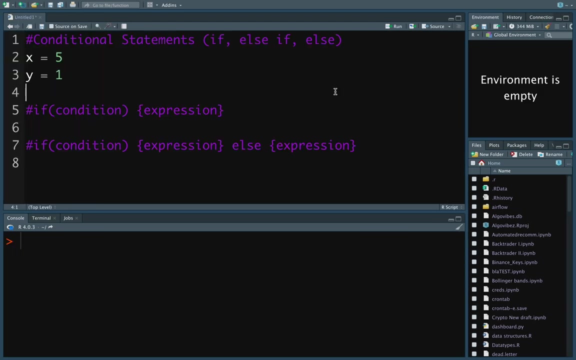 to calculate the average score De Niro is getting for his movies. I could use the mean function, then take the second column here, Right, And with that I'm getting the the average score. Okay, so let's move to part three. 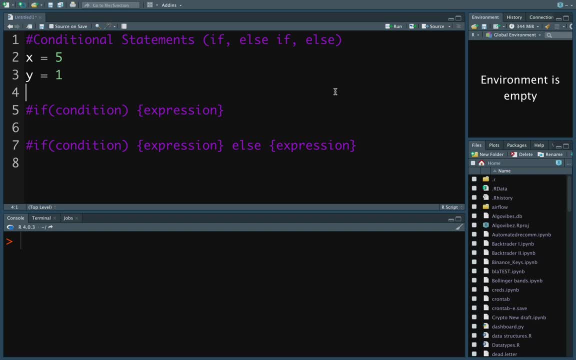 the control flow of R And we are starting with conditional statements. So if else, if and else. So we have those two variables here, Let's execute them, And we just want to check if X is larger than Y And if that's the case, 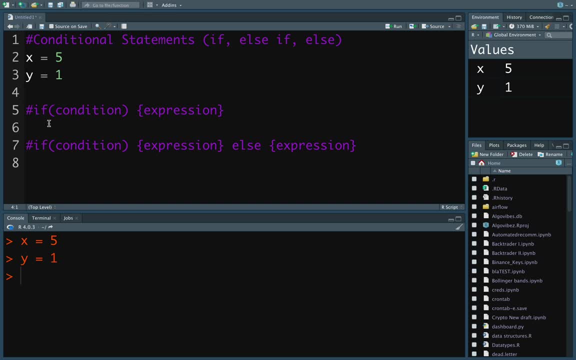 we just want to print out: X is larger, Right? Therefore we can use an if condition, And you are seeing the syntax here. So if then in parentheses a certain condition is fulfilled, then I want to get the expression here. So this is just. 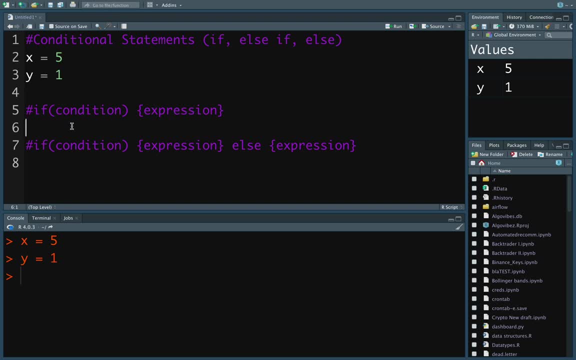 what has to be done if the condition is fulfilled. So let's actually do that. Let's say, okay, if X is larger than Y, then open up curly brackets. We want to print out: X is larger, Right? So if we are executing that, 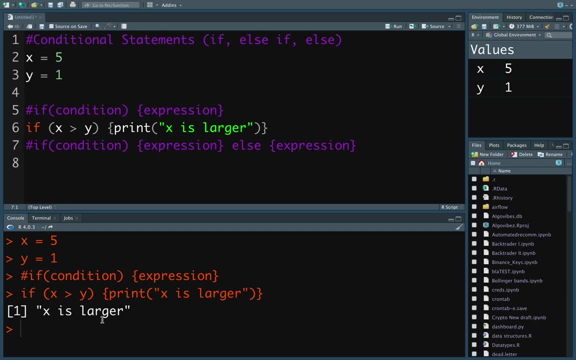 you see we are getting the output: X is larger. Right Now, if I'm changing the sign here and say, okay, X is smaller than Y and execute that, I'm getting no output here Because this condition is not fulfilled, Right. 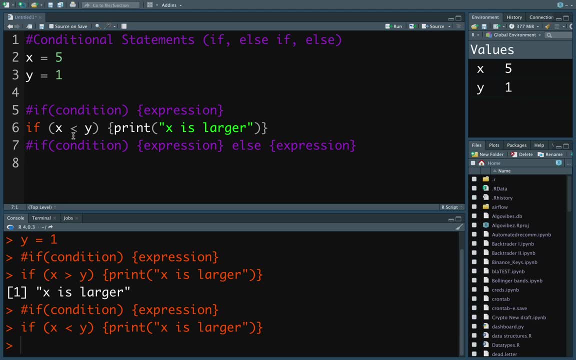 But I didn't tell R what to do if this condition is not fulfilled And therefore I can use the else statement here. So let's copy paste that And then define else And just state what should be done if this condition is not fulfilled. 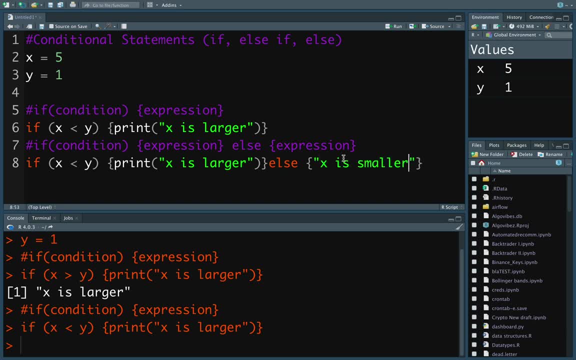 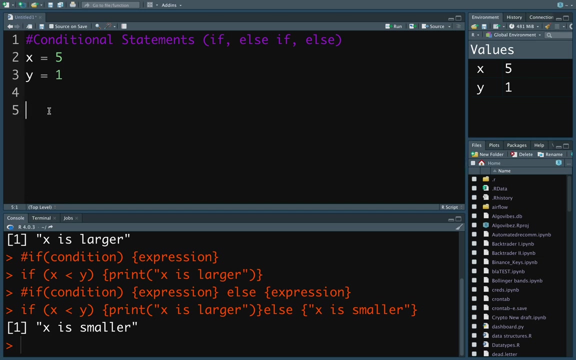 So we are just saying X is smaller. So you see, here X is smaller now, Right Now. I want to also cover else, if. But therefore we have to get rid of that all here and set up a whole if else construct. 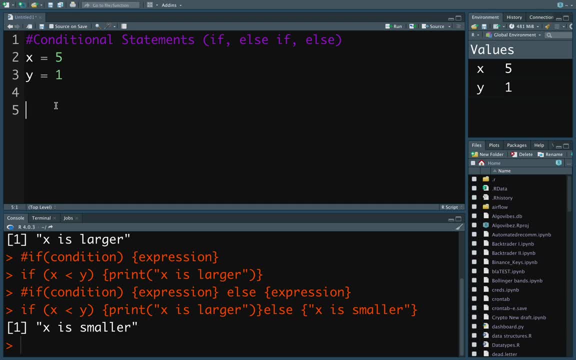 And there are some things which have to be taken care of. So, first of all, we are defining an if condition here And we are staying at if X is larger than Y. If that's the case, I want to print out: X is larger. 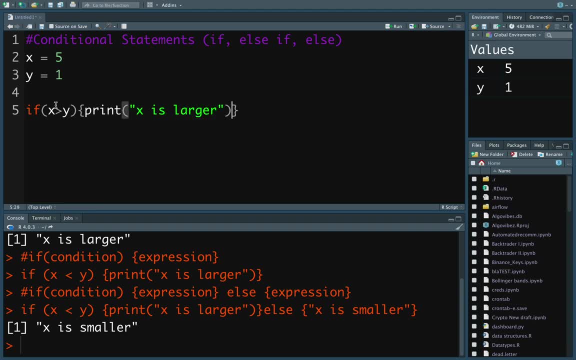 Right Now the else if statement I want to write into the next line, And this is kind of tricky with R. So if I would write else, if here this wouldn't work, because this line is being executed and R is like: 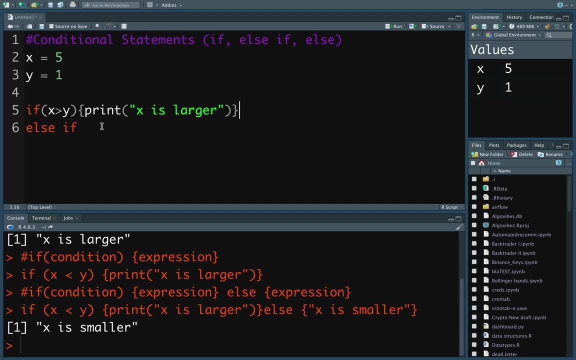 okay, this is done And it wouldn't recognize else. if So, I'm just showing you. So let's just take the opposite here. If X is smaller than Y, we are printing out. X is smaller, So let's execute this, or let's execute this whole script. 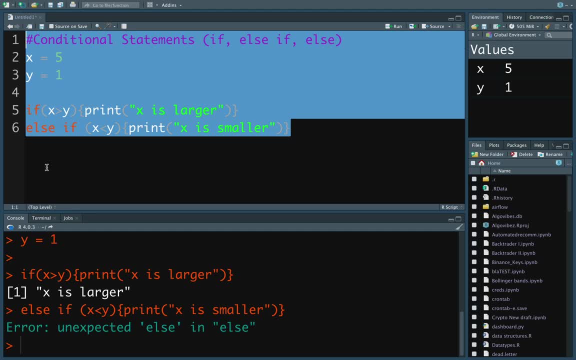 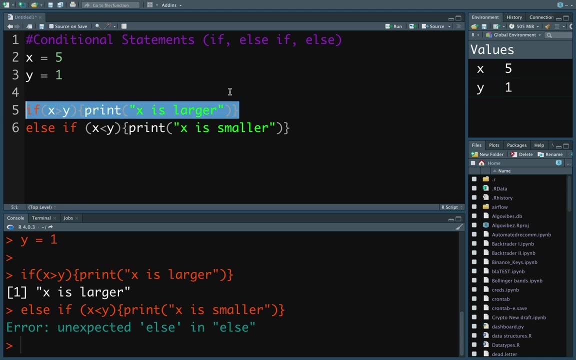 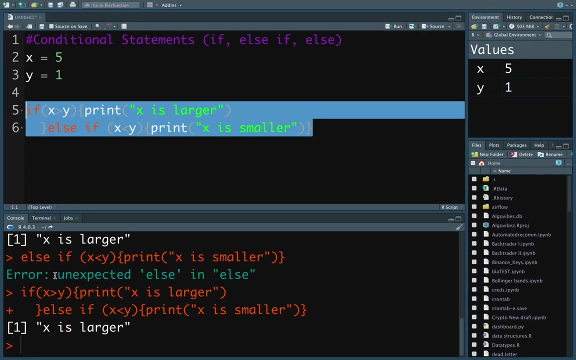 Now we see unexpected else in. else Because R isn't recognizing this. else because the if statement is already done. So how can I solve this problem? By just setting this closing curly bracket in the next line and set the else if behind that. So if I'm executing that again, 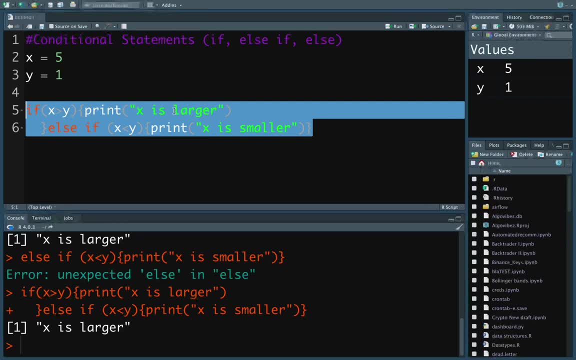 you see this is working. So this is really important, right? But anyhow, we have defined that here. But I actually wanna do something else here, And that is I wanna check if X is equal to Y as the else if statement here. 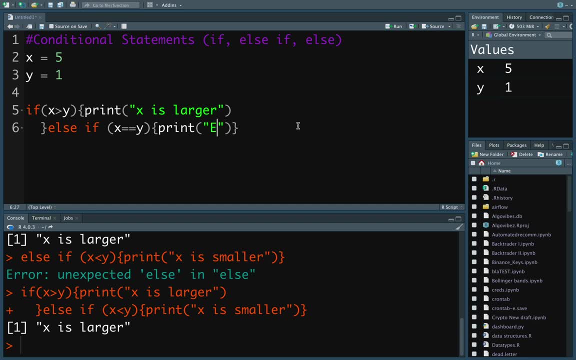 Right? And then say equal or equals, And in the end the else statement should contain X or smaller. These are the three possibilities, right? So again, I'm setting the ending curly bracket in the next line until R to print out X is smaller. 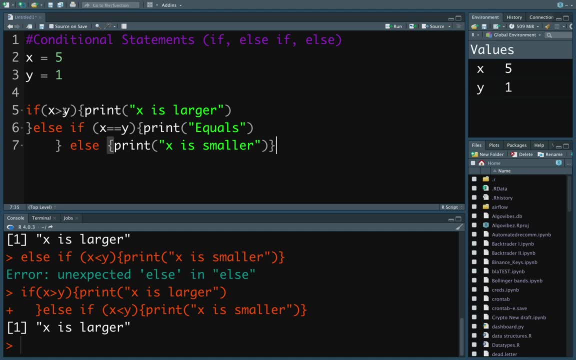 Right. So we have three possibilities: X is larger than Y, X is equal to Y, And if none of these are the case, X must be smaller than Y. Right Now, let's execute that for this script. And, of course, X is larger as. 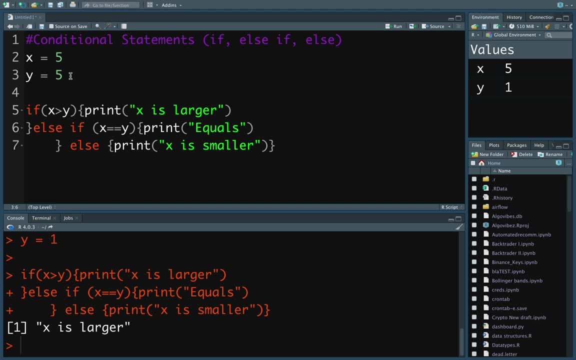 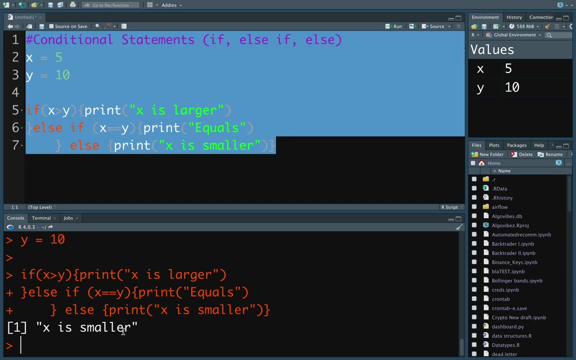 X is five here. right, Let's change Y to five, so the numbers are equal. And if we execute that, again we are getting the output that the numbers are equal. right, And let's say Y is larger than X, Then we are getting the output that. 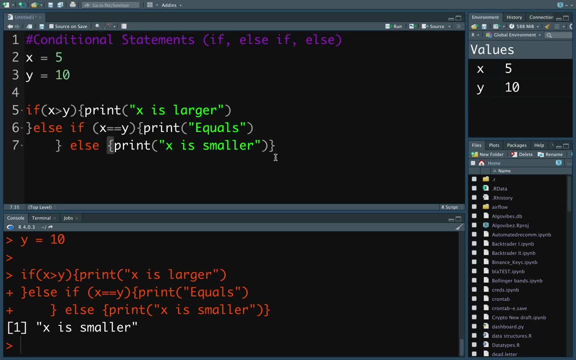 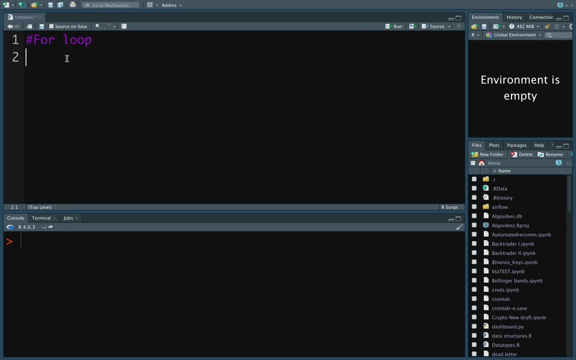 X is smaller. So this is how conditional statements are working. Okay, so let's move on to loops, and we are starting with the for loop. The for loop is just an iteration over a certain sequence, So let's take an example. We are using the for keyword. 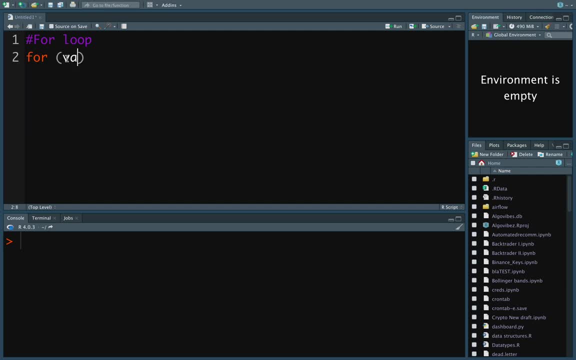 and then specify the element which I'm just calling value in a certain sequence. So let's just take one to five And here in curly brackets I'm specifying what to do in each iteration And if I'm printing out the value. 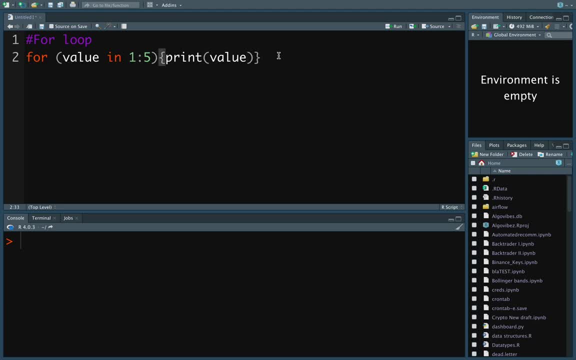 which is the element in this sequence. I'm just getting all values from one to five here, Right? I could also, by the way, I could also call that I and this wouldn't change the result here, right? So this is just the element. 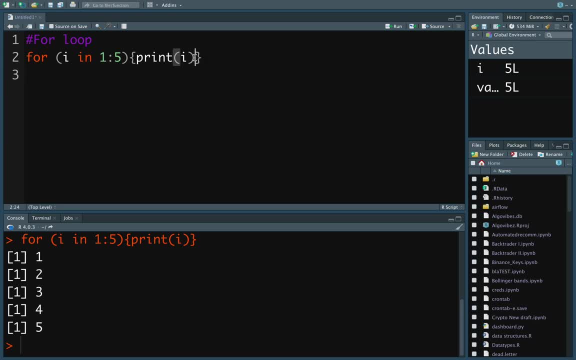 in the sequence one to five. I could also print out hello here and I will get five times hello, as in each iteration. so the hello statement is printed out. So in each iteration, from one to five, we are printing out hello. You could also. 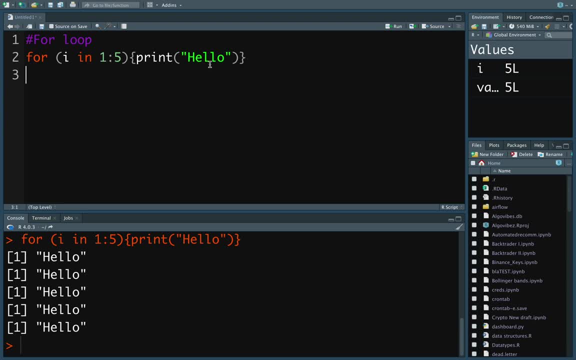 incorporate conditional statements here in the for loop. but we are doing that in the fizzbuzz task anyway, so I'm not covering that. What I also want to cover here is: you can also iterate over vectors. So if we are creating a vector here from one to 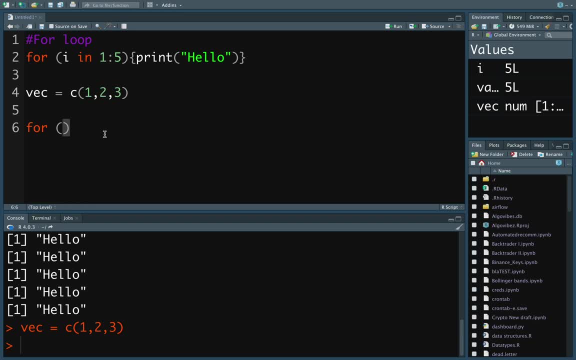 three, and use for value in vector and we are printing out the value. we are just getting the elements in this vector. You can iterate over all data structures, so matrices, lists and so on. Okay, so let's move on to the while loop. The while loop is a. 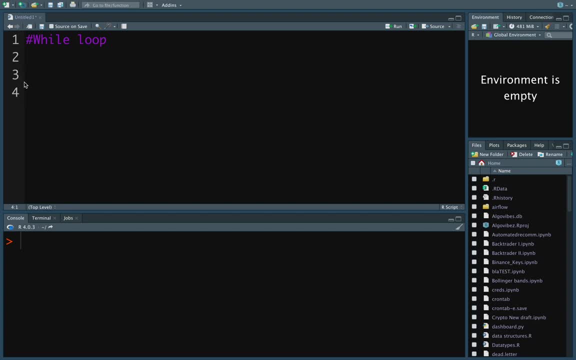 loop which is running until a certain condition is fulfilled. So let's take an example. Let's say we have an initial value here, which is one, and we want to print out this value as long as this value is smaller than five. but we want to increment. 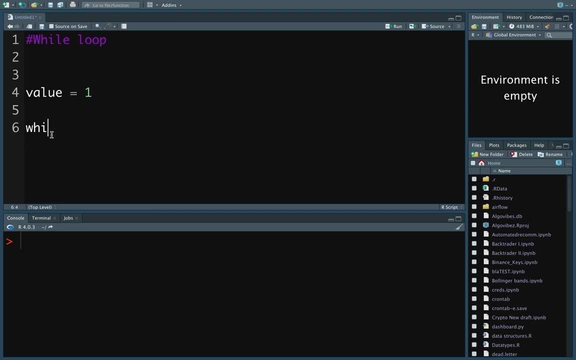 the value in each iteration. Therefore, we can use a while loop. So while this value is smaller than five, we want to print out this value and after that we want to also increase that value by one Right? so if we are executing that, 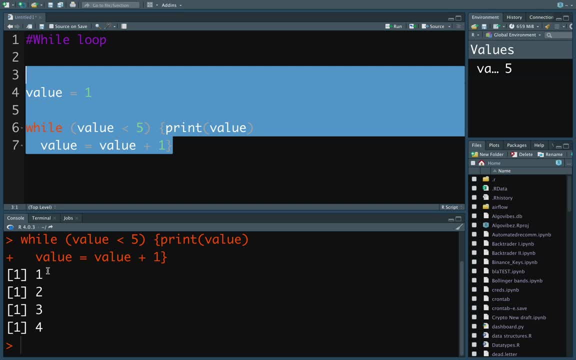 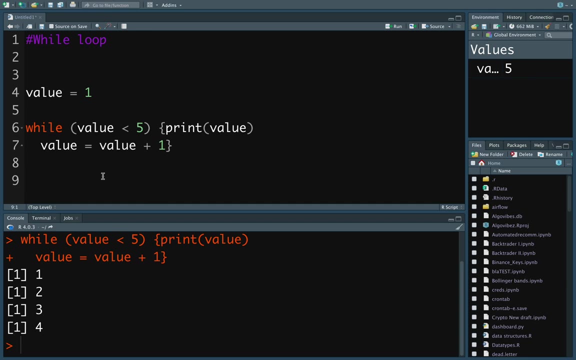 you see, we are getting the value until it is five, Right? so as long as it's smaller than five, we are getting the value here. You can also run infinite loops by just providing while and then true or t whatsoever, and then you can print. 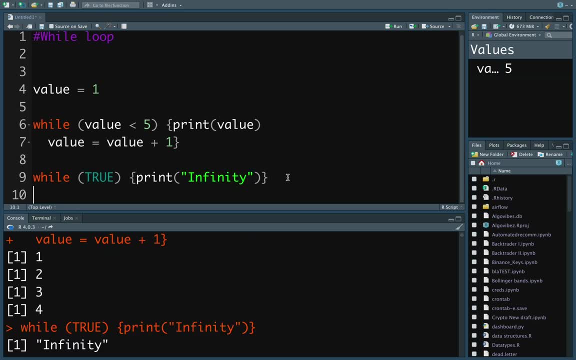 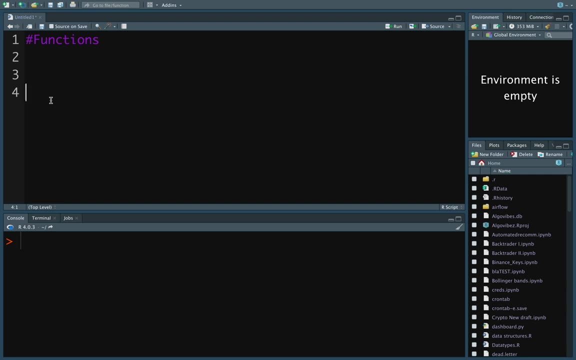 I don't know infinity, and with that you are getting an endless loop here. You see, this is being printed out until the end of time, So I'm manually stopping that. Okay, so let's move on to functions. Functions are just performing a certain 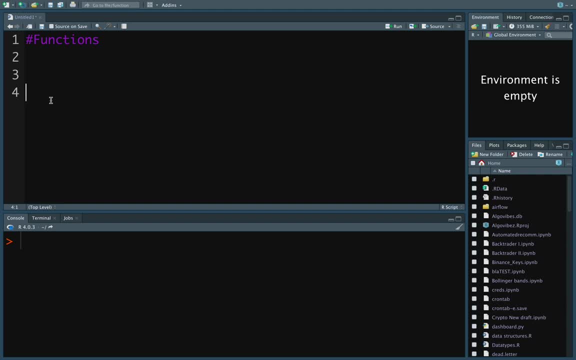 task. You can call them whenever you need them, and you can also provide parameters to these functions. Creating functions in R is, at least in my opinion, pretty extraordinary, because you have to store them in variables, But nevertheless, let's start easy. 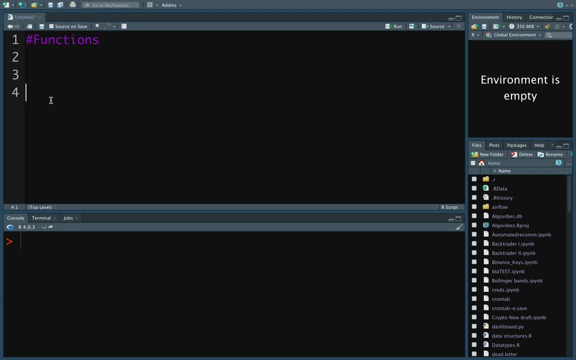 So let's start with a very simple function which is just printing out hello. Therefore, I'm using x as the variable where I'm storing the function in, Then use the function keyword and take no arguments. So I'm just using empty parentheses here. 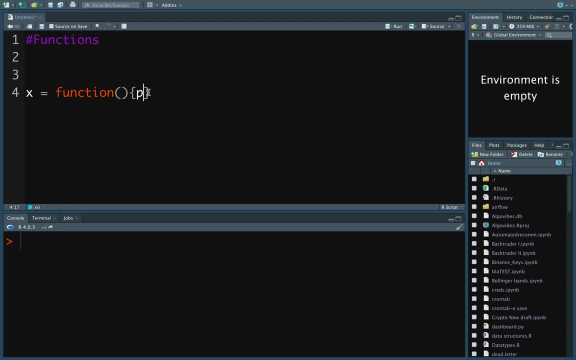 After that I have to define what has to be done inside the function And, as said, I just want to print out hello. So we can execute that and call this function by typing in x and then use these empty parentheses And you will see that. 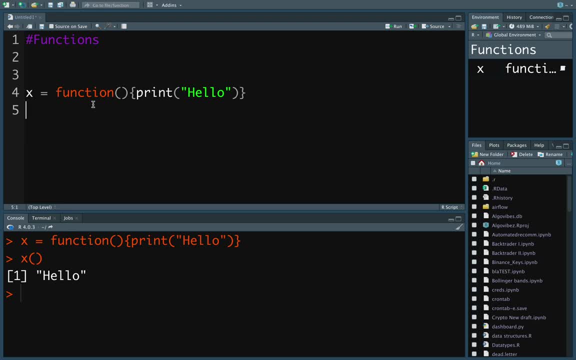 hello is being printed out, Alright. The second function is taking an argument. So we are just defining y here and take arg1 and in this area. so what has to be done inside the function? we are just squaring our argument, right? 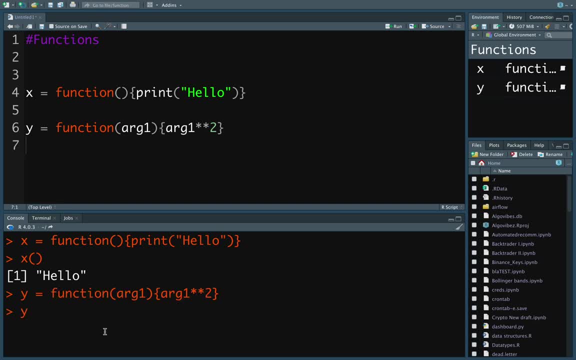 So let's execute that. and if we are providing- I don't know- two, we are getting four. If we are providing 25, we are getting 625, and so on. Last but not least, we are defining- yeah, let's call it- a more complex function. 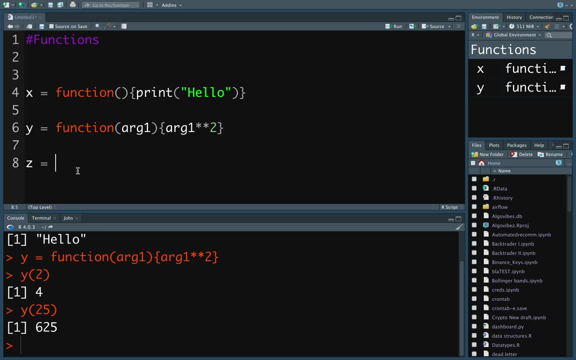 which is not really the case, But this is containing some more concepts here, So we can take function again. Now we are taking two arguments here And inside this function now we are defining a local variable which is not popping up here, because this is: 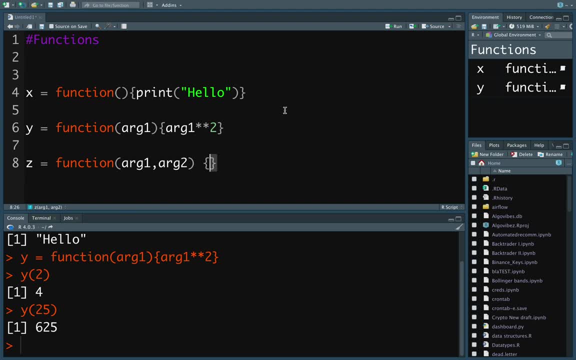 only defined inside this function and it's not defined on the global area, So inside the script. So let's call that log for local variable and this is just adding up the two parameters right And after that I want to return this local variable. 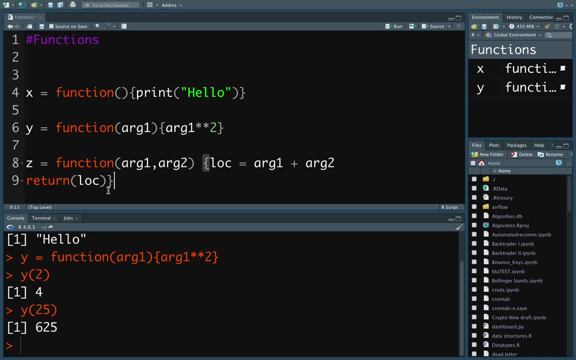 to get it on the global area, Right? So when I'm calling this function, I'm getting this local variable. So if I'm executing that, and let's just provide 10 and 10, so the local variable should be 20 in this case, right, I'm getting. 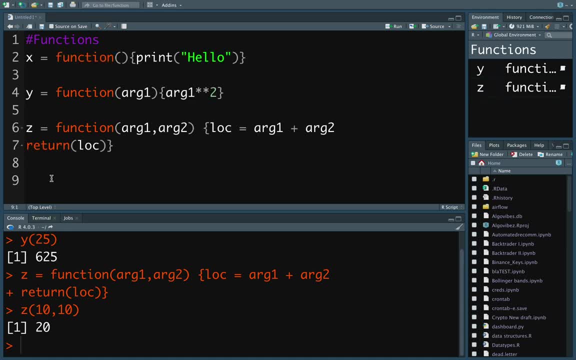 20 here, Okay, Okay. so let's apply some knowledge we have attained until now by coding a recursive function and, specifically, a factorial function. So if you want to take a challenging task, you can pause the video now. So we are coding a recursive function. 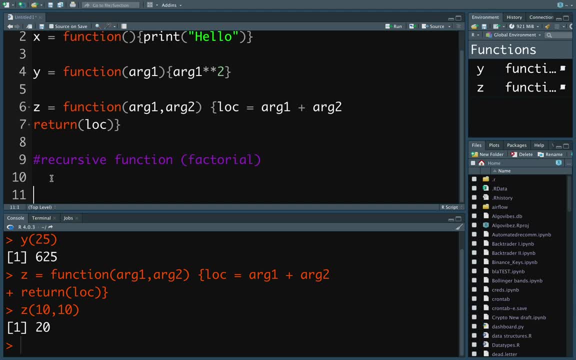 and we are taking a factorial here. So first of all let's call that factfoo and we are defining a function which is taking n as the argument. So this is just any number where we are getting the factorial for right. So first of all we have to specify: 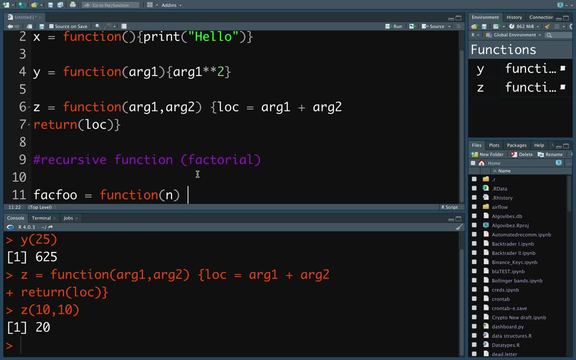 what is happening if n is 0 and the factorial of 0 is defined as 1.. So we have to specify that with an if-condition here. So if n is equal to 0, we want to return the 1 here, Right? 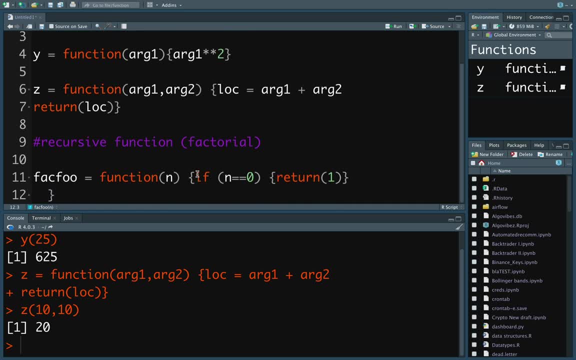 Perfect If that's not the case. so we have a higher value than 0, so we are just taking else. here we want to return the function value, but for n minus 1. And after that we want to multiply that by n. 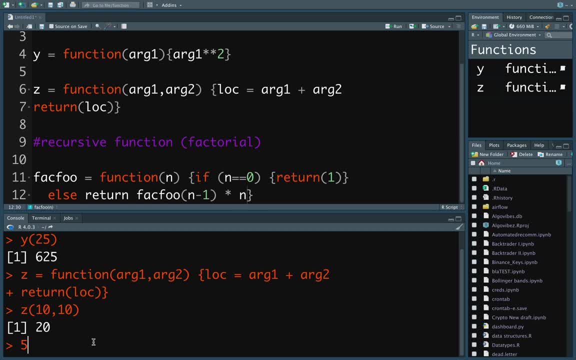 So why is that? Because, as you might know, a factorial is working like that: 5 times, 4 times, 3 times, 2 times 1 here. right, So that's already it. I think I forgot the parentheses here. Yes, I did. 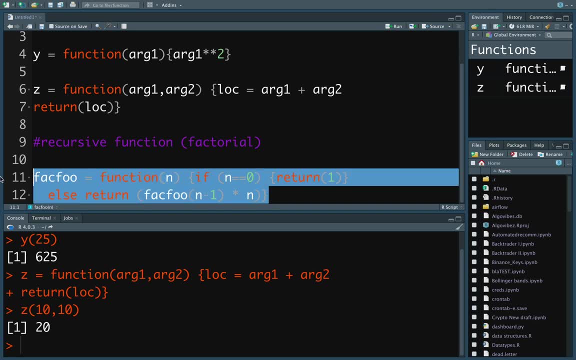 So this has to be in parentheses And if we are executing that we can try out if everything went well. So factorial of 5 is 120. Works. Factorial of 0 is 1.. Factorial of 10 is this number here. 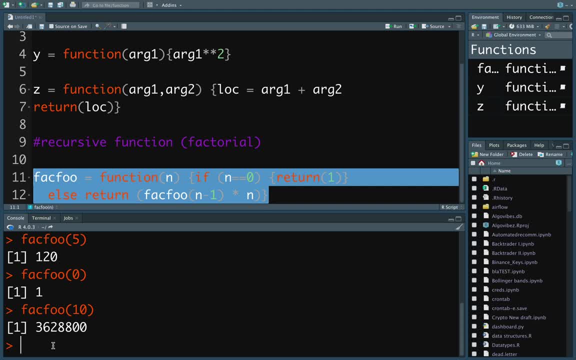 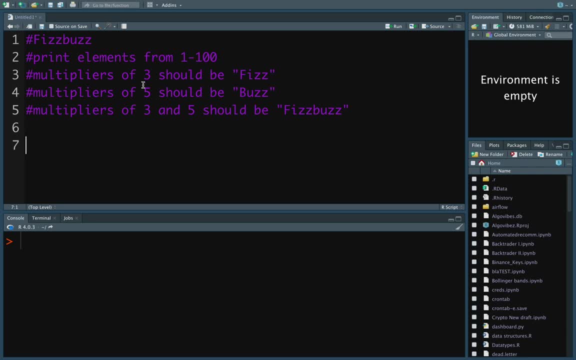 And so on. So this is a recursive function. Okay so, last but not least, fizzbuzz. So we should print out elements from 1 to 100.. Multipliers of 3 should be fizz. Multipliers of 5 should be buzz. 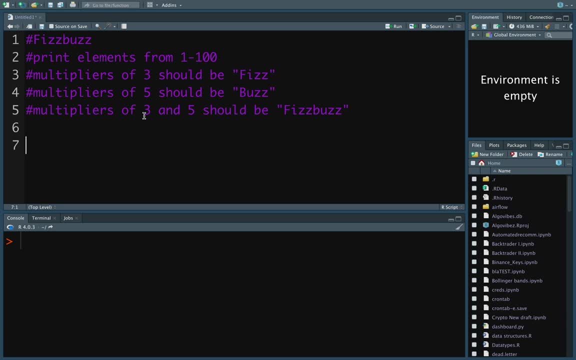 And multipliers of 3 and 5 should be fizzbuzz. So if you want to take the challenge, pause the video right now. Let's solve that. So to print out all elements from 1 to 100, the for loop is the right pick. 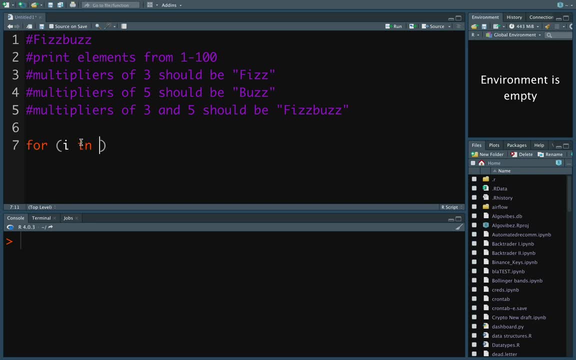 here. So we are taking for i in 1 to 100.. Now the first thing is to check for the multipliers of 3 and 5. So we are using an if statement here And check if the modulus of 3 is equal. 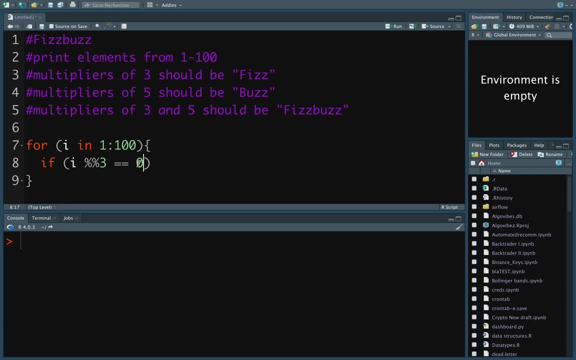 to 0.. So I've explained that in the beginning, right? So if that's 0, we have a multiplier. Now we are using something which I didn't cover, which is the logical operator and Which is just enabling us to check for. 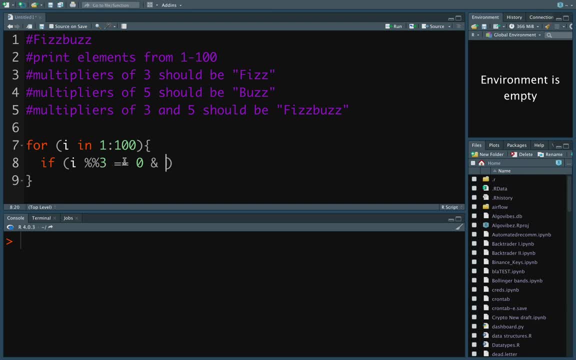 multiplier conditions, right. So to check for that. and another condition which is fulfilled. So the other condition is, of course, the modulus of 5, also equal to 0 here, right? And if that's the case, we want to print out this bus, right? 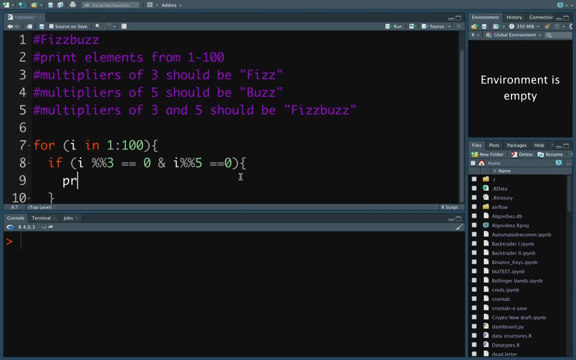 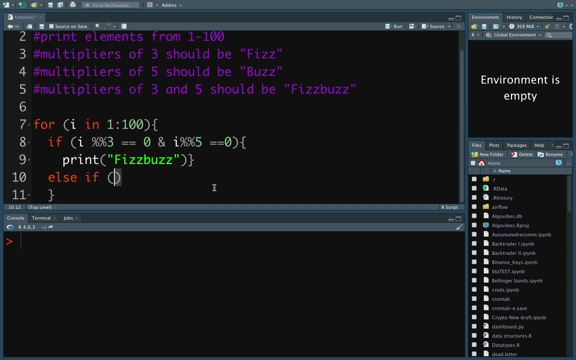 So print this bus. So let's close the parentheses here And get rid of the. this one should be here, Okay, First condition: Second: one multiple of 3, which should be this right, So we are taking else, if i modulus. 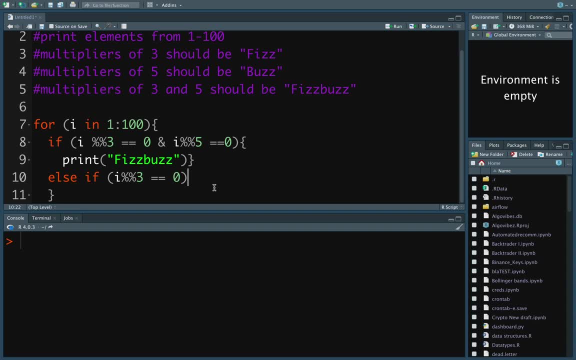 3 equals to 0. And then we are printing out this, Print this, And next one is the modulus of 5 equals to 0.. I want to print out bus here. And, last but not least, we just want to print out. 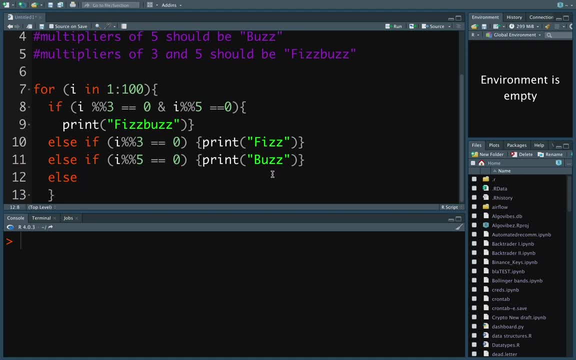 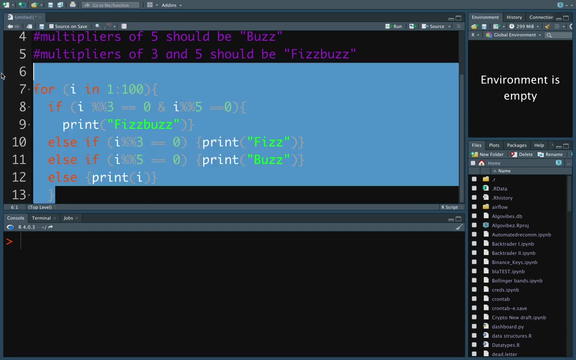 the number right, So we are using else and then print i. So do we have the parentheses right? Yes, I do. So let's test that by executing that. And now we see we are getting what we wanted to get Right, So let's do some quick.